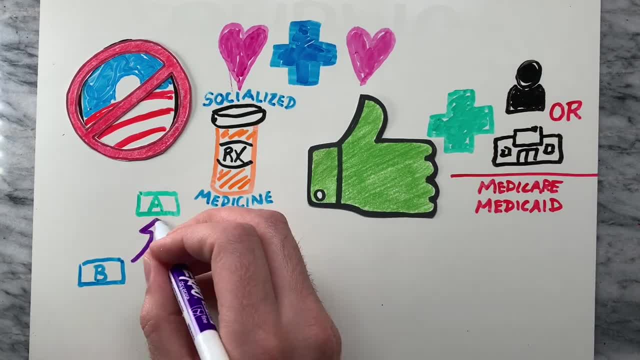 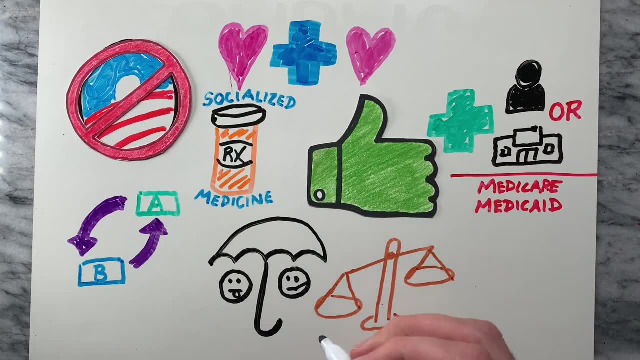 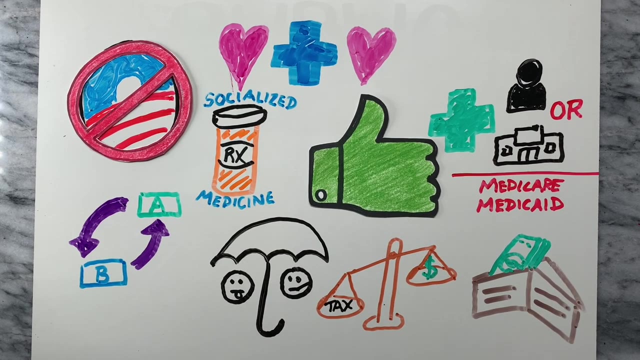 or Medicaid for low-income families. Many Republicans support increased health insurance portability, laws promoting coverage of pre-existing medical conditions and tax benefits aimed to make health insurance more affordable for the uninsured and to promote universal access. When it comes to education, most Republicans support school choice through charter schools. 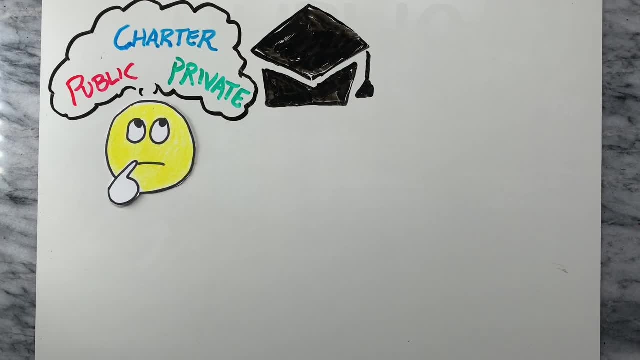 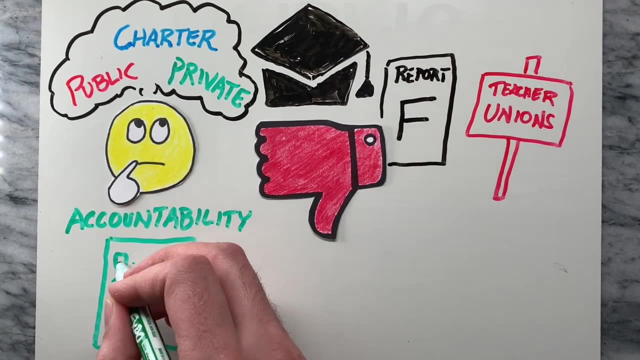 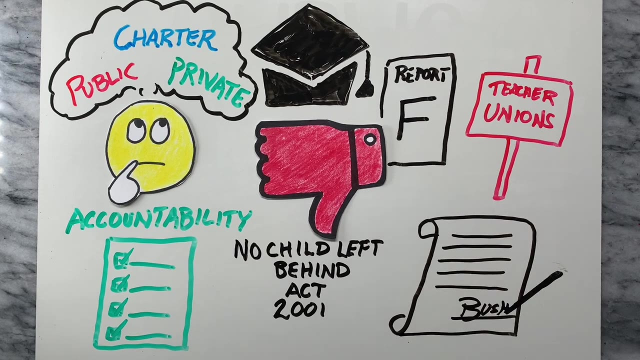 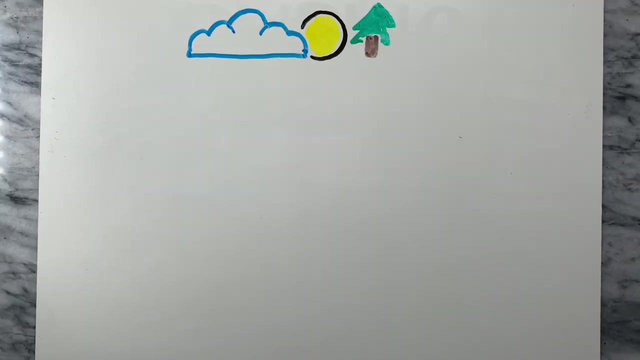 and school vouchers for private schools. Many have denounced the performance of the public school system and the teachers' unions. The party has insisted on a separate school system for private schools. The party has insisted on a separate school system for private schools. The Republican Party, led by President Richard Nixon, is most prominent in the 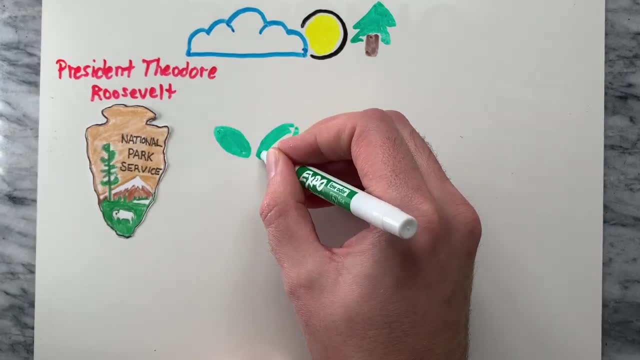 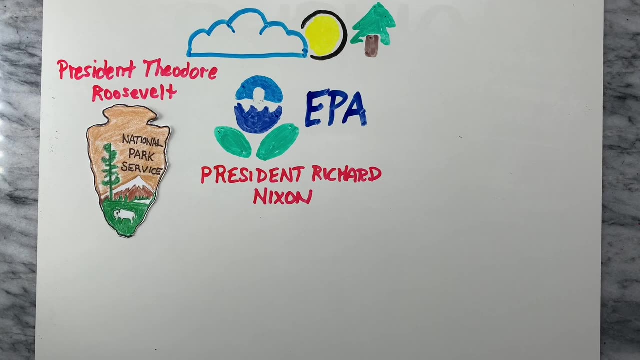 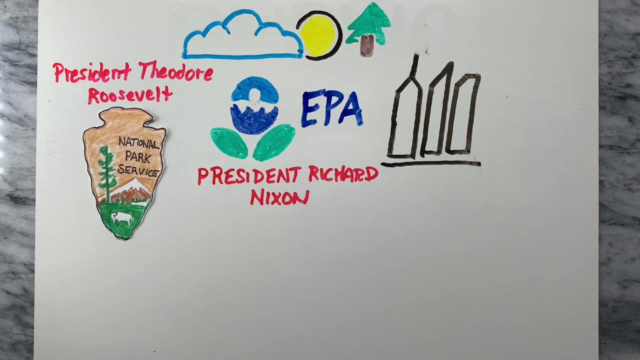 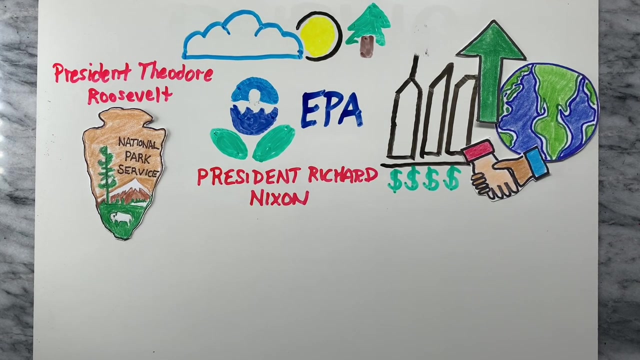 no-child-left-behind act of 2001.. Protection Agency in 1970, and in 2000,, the Republican Party adopted, as part of its platform, support for the development of market-based solutions to environmental problems, stating that economic prosperity and environmental protection must advance together. 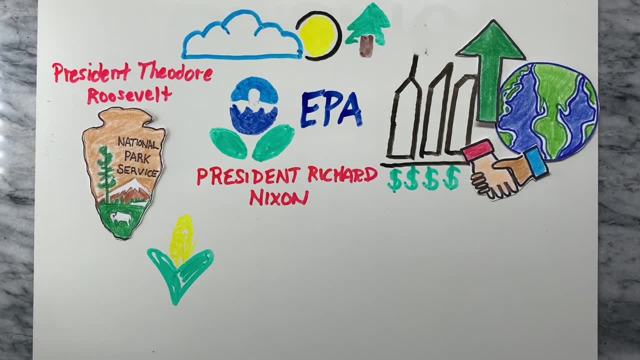 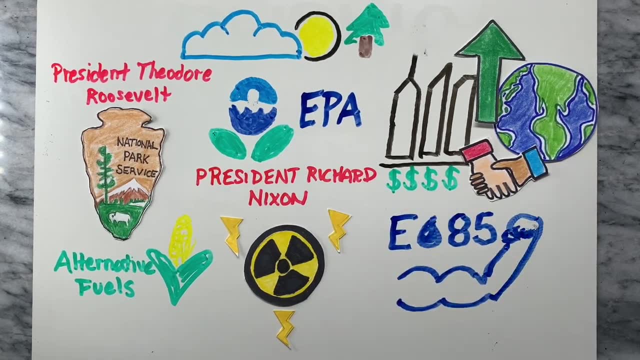 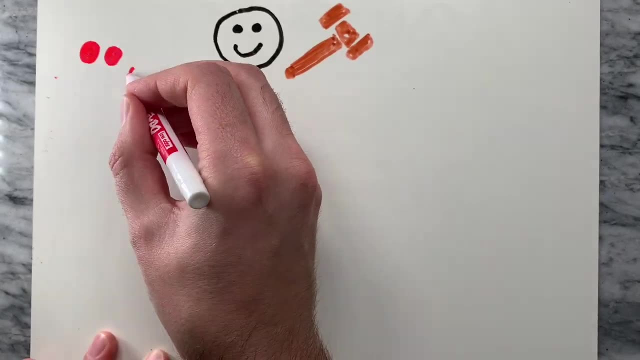 Many Republicans have supported increased federal investment into the development of clean alternative fuels, increased nuclear power, as well as fuels such as ethanol, as a way of helping the US achieve energy independence. The Republican Party has generally been associated with socially conservative policies that include: traditional family values, often rooted in Christianity, although there are factions that are more liberal in their views. As of 2022, a majority of Republican voters support same-sex marriage, with public opinion within the party changing substantially on the issue in recent years. 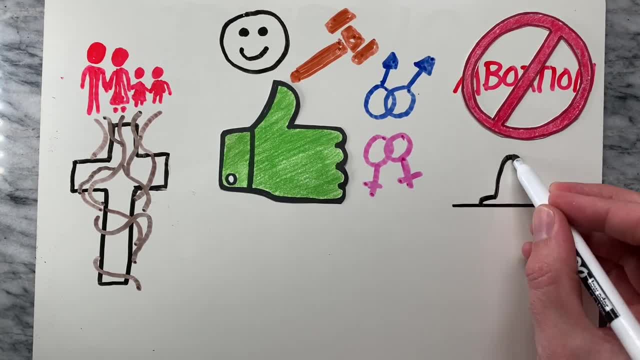 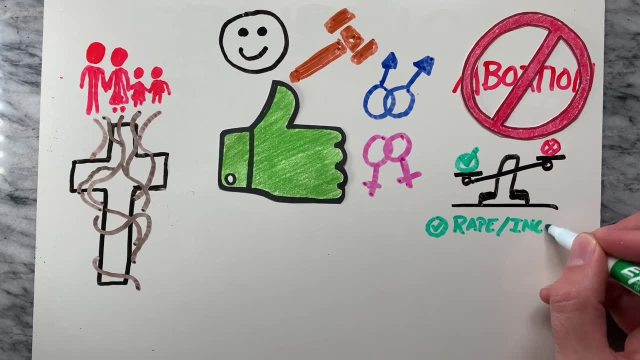 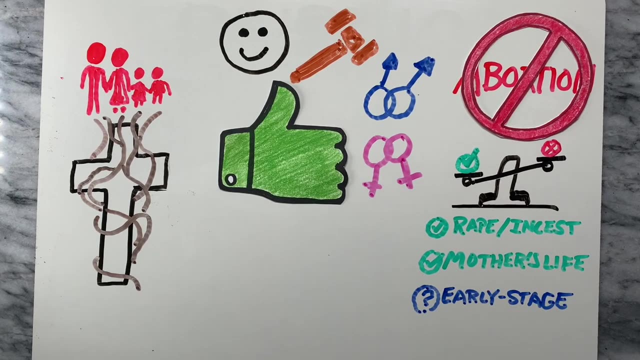 A majority of Republicans are, at the very least, moderately anti-abortion. They oppose elective abortions on religious or moral grounds. However, many hold exceptions in the case of rape, incest or the mother's life being at risk, while others may accept early-stage abortions. 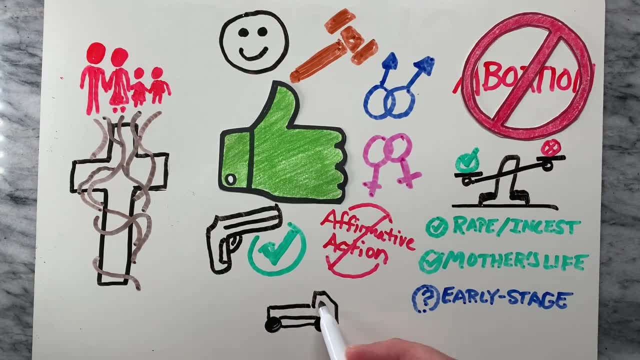 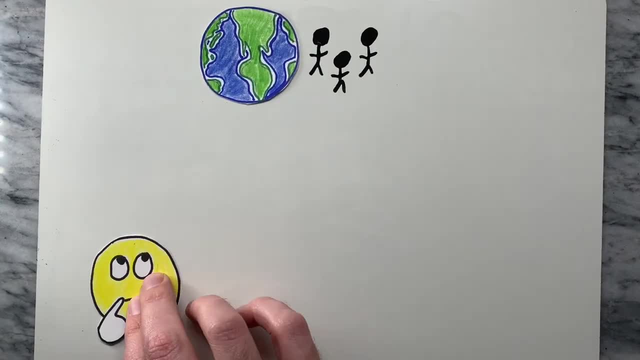 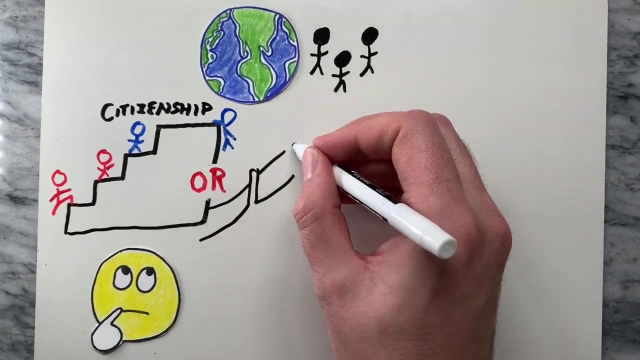 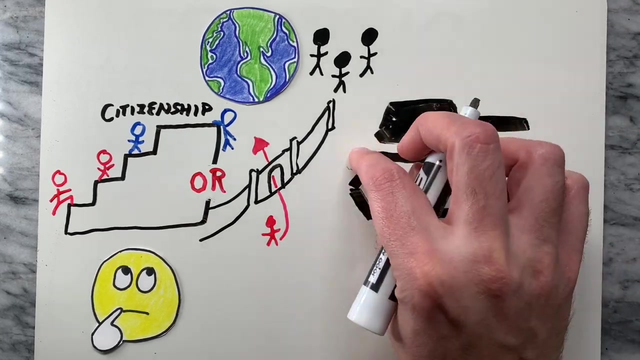 Most conservative Republicans also oppose gun control, affirmative action and illegal immigration. Republicans are divided on how to confront illegal immigration, between a platform that allows for migrant workers and a path to citizenship for undocumented immigrants. Republicans in general tend to be more pro-military than the Democratic Party. however.